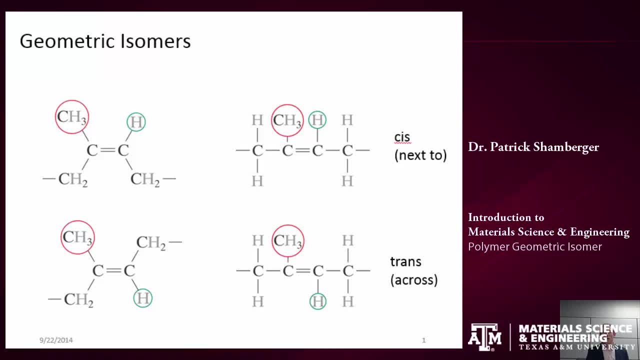 have important effects on the properties of those polymer chains. So geometric isomers are referring to different, unique arrangements of side groups within an individual repeat unit. So let's look at an example of some of these. In this case we have two different kinds of side groups. We have propyl groups, which are composed 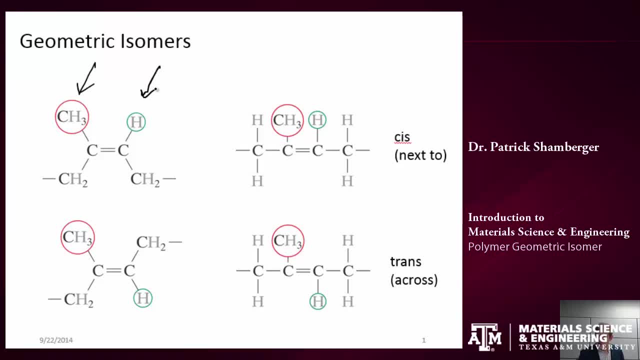 of a carbon with three hydrogens coming off it And we have a single hydrogen atom as a side group. Now you'll note that there is a double bond between those two carbons, And that's really important. It's become clear why momentarily. 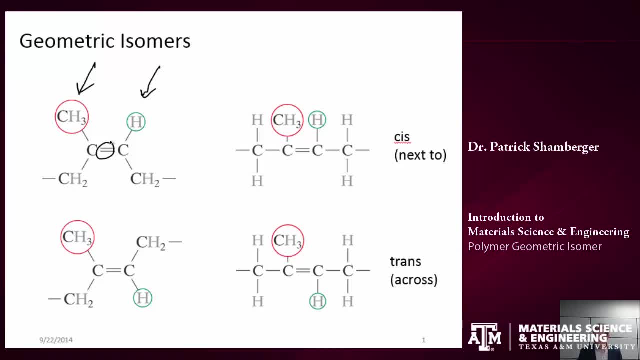 So we can have two different kinds of arrangements of these side groups. We could have what's called the cis arrangement, whereby the propyl group is next to the hydrogen group, Or we could have the trans arrangement, whereby the propyl group is diagonally across that. 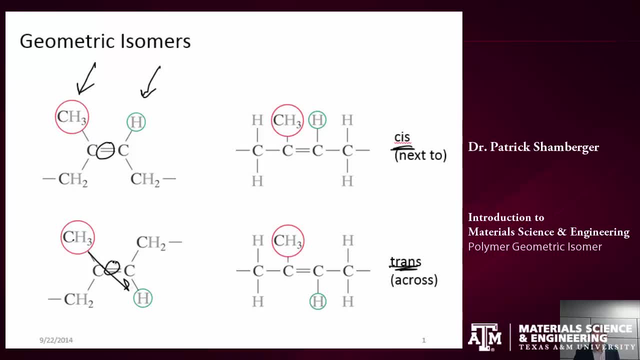 repeat unit from the hydrogen group. Now it's important that you have a double bond because that is what creates a stiff backbone and stops that backbone from rotating. And you need that stiff backbone because if you rotate, then you can go back and forth between 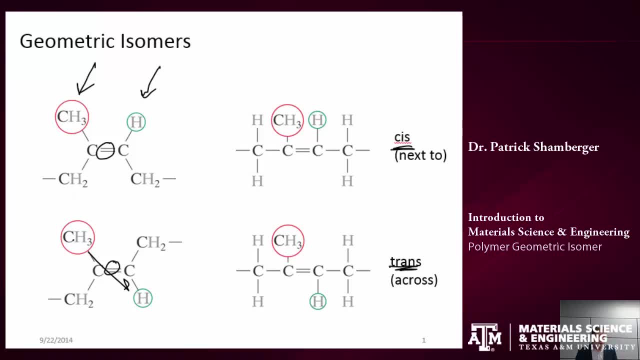 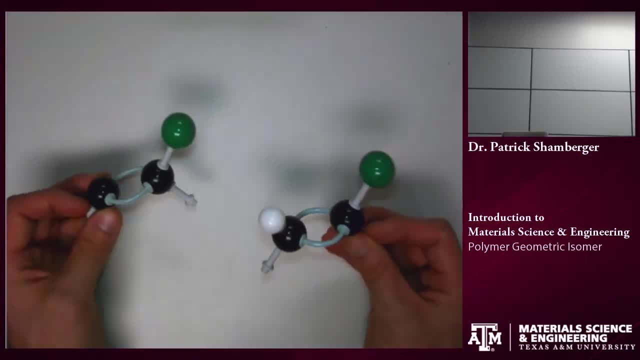 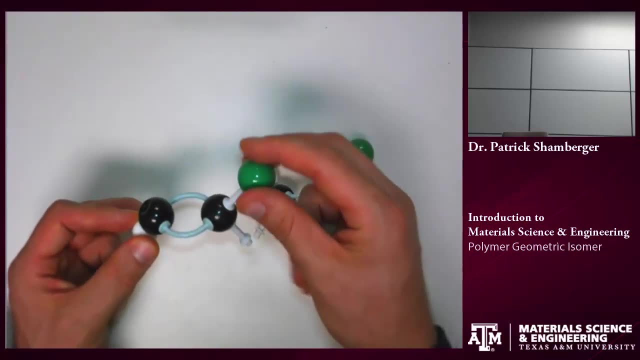 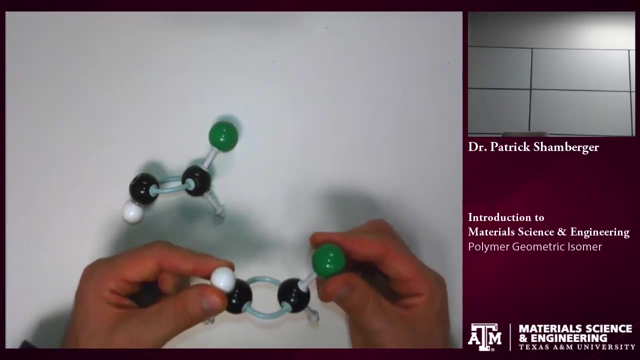 that cis and trans configuration. So let's look at a couple examples on a 3D model. These are two different repeat units. In one case I have the trans configuration, So this side group is diagonally across The repeat unit from this side group. In the other case I have a cis configuration. So 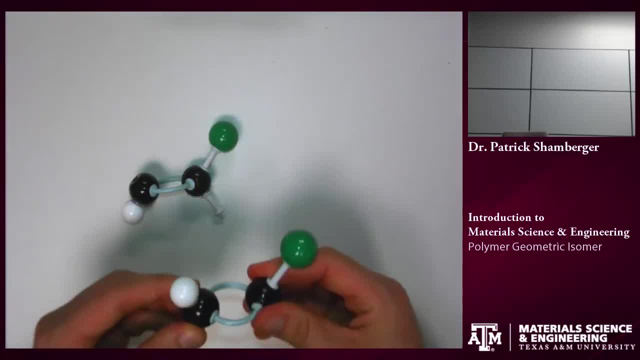 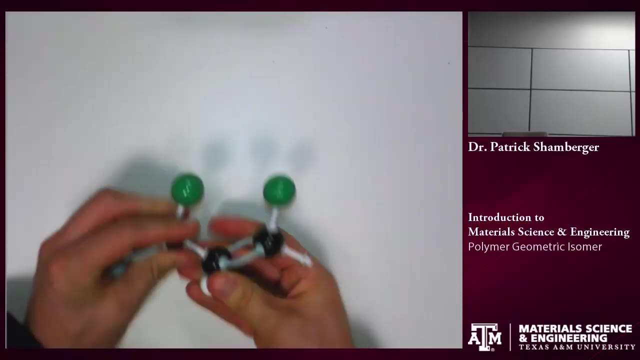 these two side groups are next to each other. Now there's no way to rotate this, to go from one case to the other, because that's a double bond And, remember, double bonds don't allow for free rotation along those axes. So I could form a polymer chain by combining a bunch of different ones And typically 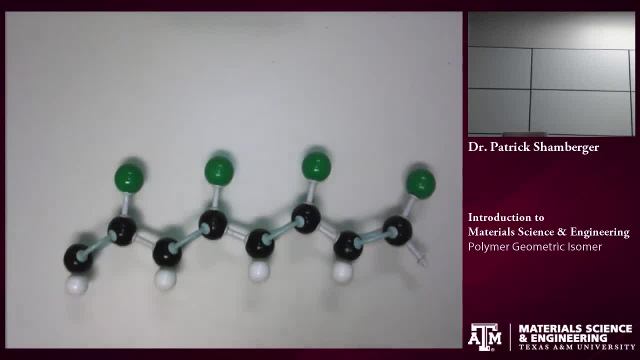 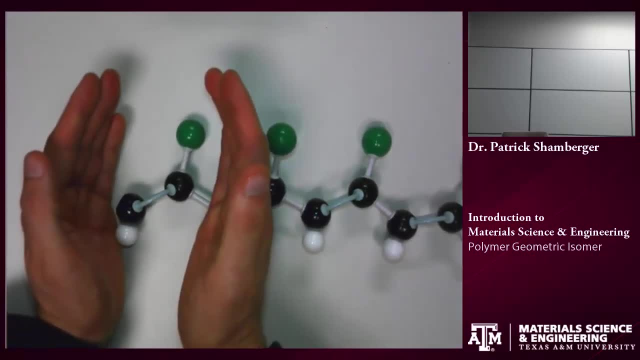 during the synthesis process. So I could form a polymer chain by combining a bunch of different ones, And typically during the synthesis process we're either using cis or trans configuration type repeat units. So this is a polymer molecule that's composed of repeat units in the trans.